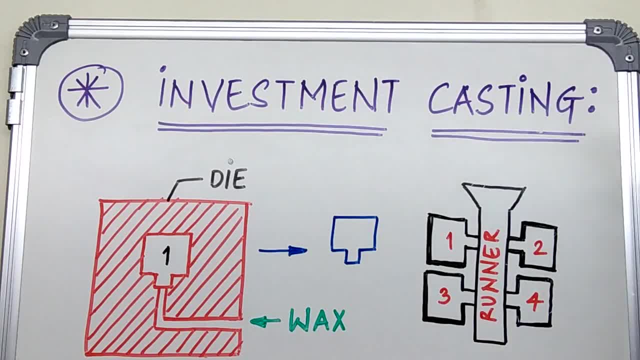 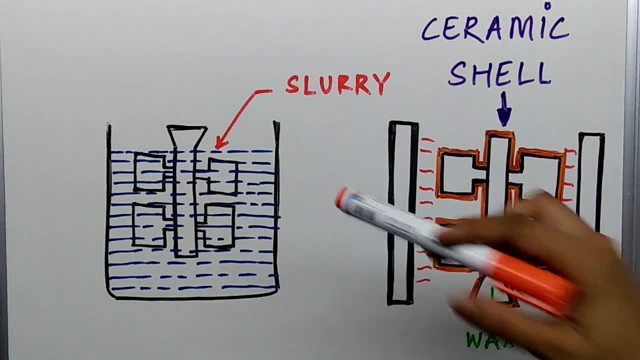 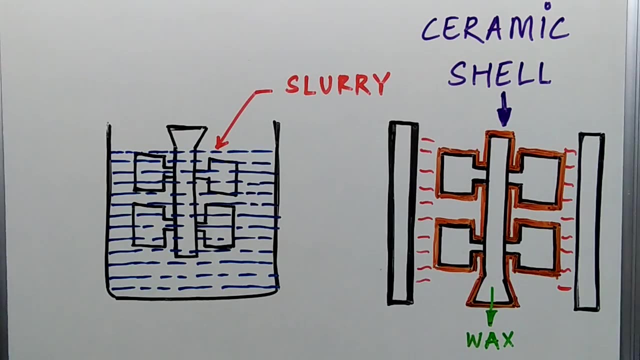 And this is the pouring cup through which we will be pouring our molten metal. Now, once the runner assembly is made, there is this slurry tank in which it is dipped. The slurry tank consists of silica floor, ethyl silicate and water, and some binding acids as well. 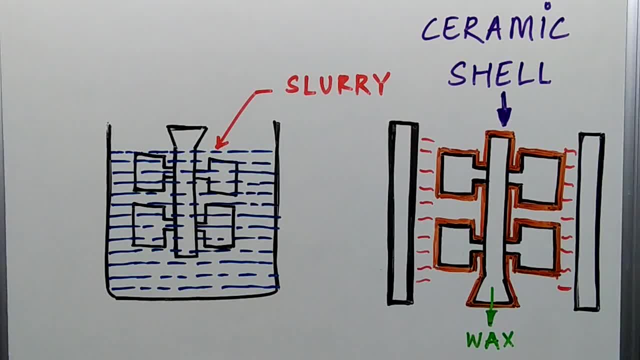 So this runner assembly is dipped into this slurry tank Three or four times, until and unless the desired thickness of the shell is attained. Once the desired thickness is attained, it is coated with very fine grains of ceramic, And then what we get is this shell which is coated with ceramic. 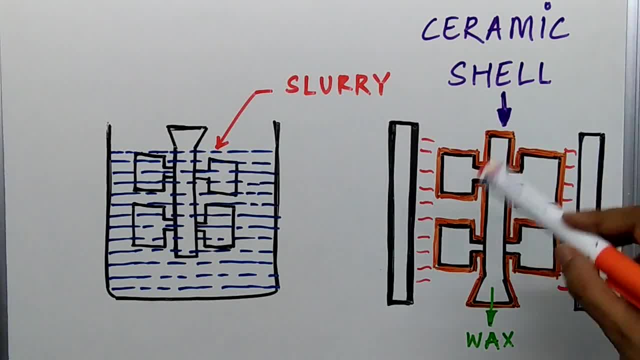 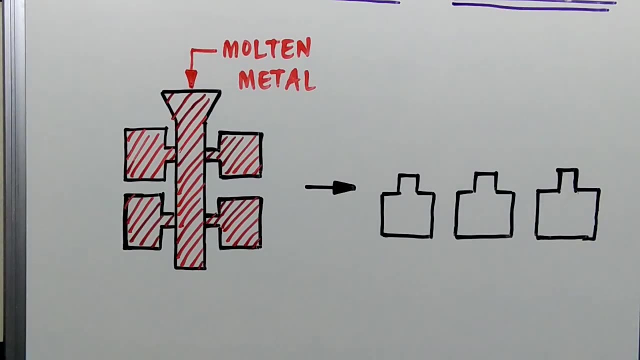 So afterwards, this shell is then heated in order to remove the wax, and the liquid wax comes out through the pouring cup. So, once we have removed all the wax from the ceramic shell, we then proceed to pour our molten metal into the ceramic shell. 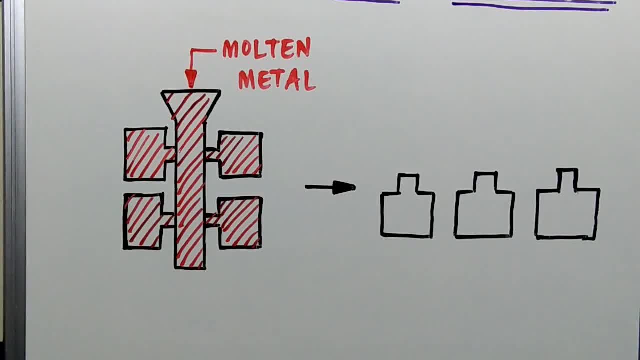 And then it is allowed to solidify for some time. After solidification process, the ceramic shell is then broken down with the help of vibration techniques, And this is the casting which we get. This is the final product which we get. So that was all about the investment casting process. 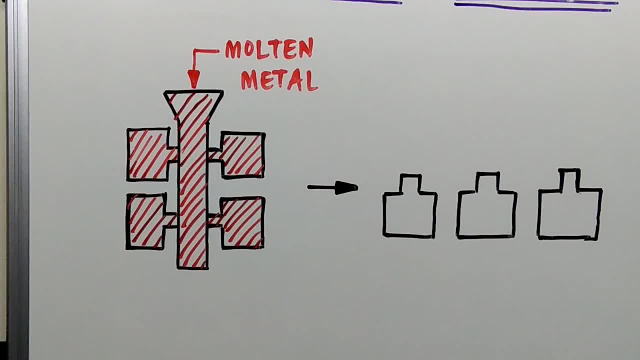 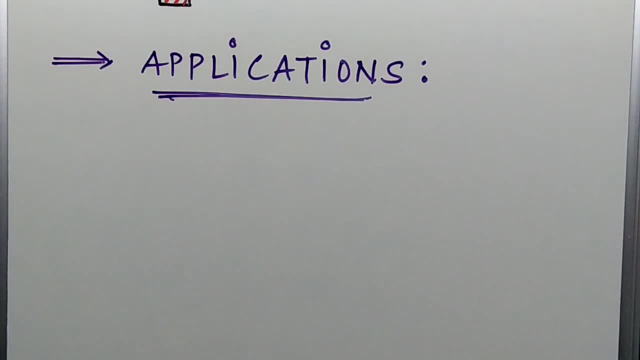 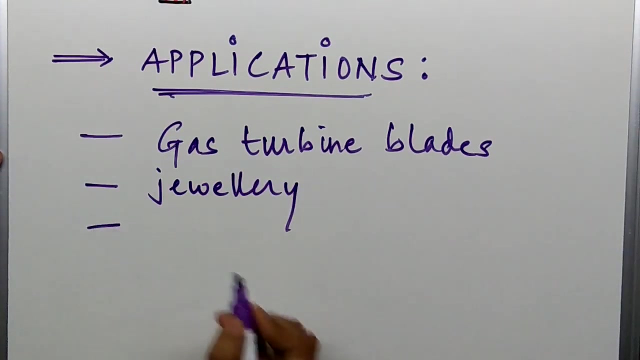 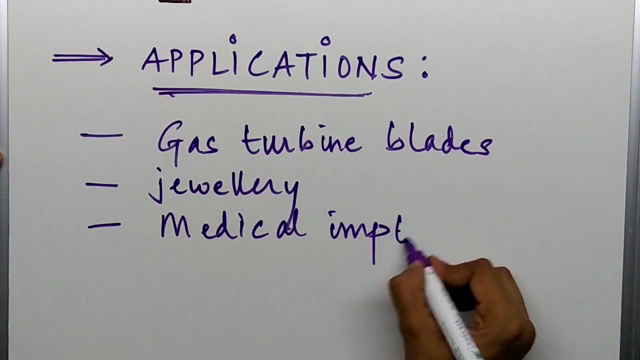 Now let's look at the applications of this process. Investment casting is usually used for small jobs, and it is used for mass production. Alright, so it finds its application in gas turbines, Gas turbines, Gas turbine blades, Then jewellery, Medical implants.